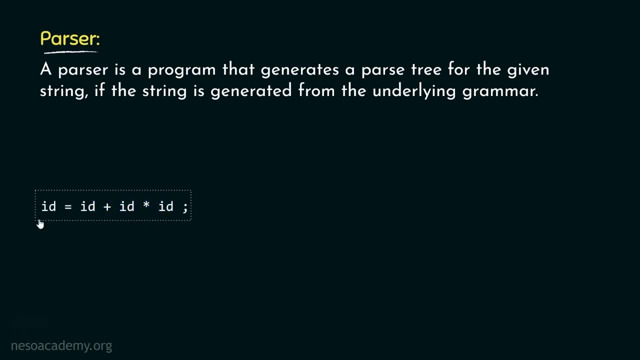 analyzer, this particular code will be converted into a string like this: Now this string will be fed into the parser, which is basically a program. Now, the job of this parser is to generate the parse tree. Now, the parse tree can only be generated if the string can be generated from. 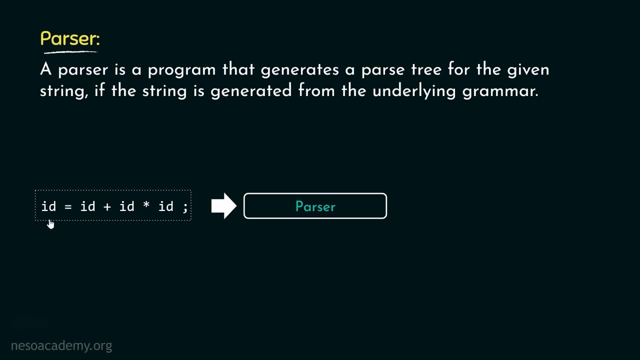 the underlying grammar. So, basically, the parse tree for this string is a string that is generated by this parser, if this particular string can be generated by the underlying grammar. So what the parser program will do? it will take the string as input and, with the help of this underlying grammar, 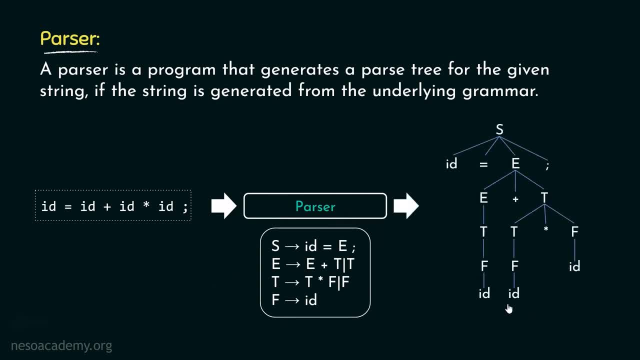 it will generate the respective parse tree. So let's revise the formal definition of parser once again. A parser is a program that generates a parse tree for a given string, if the string is generated from the underlying grammar. Let's now observe how the parse trees can be generated. Now, the generation of the parse. 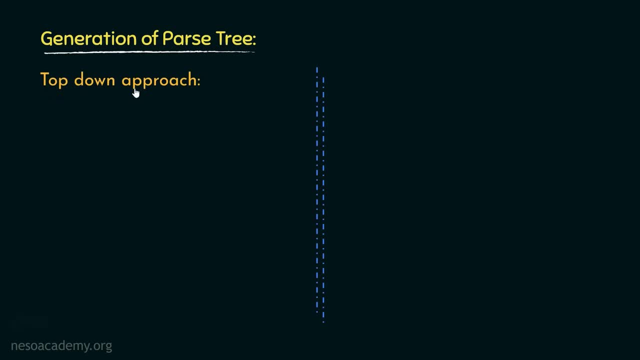 tree can be done in two ways. The first one is the top-down approach and the second one is the bottom-up approach. Now, in order to understand these approaches in bit more details, let's take an actual grammar and say: with the help of this grammar, we are to generate: 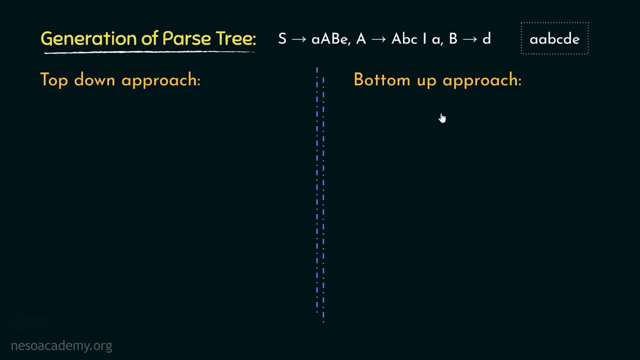 the string a, a, b, c, d e. Let's start off with the top-down approach first. Now, in case of the top-down approach, we are to generate the string a, a, b, c, d e. Now, in case of the top-down approach. 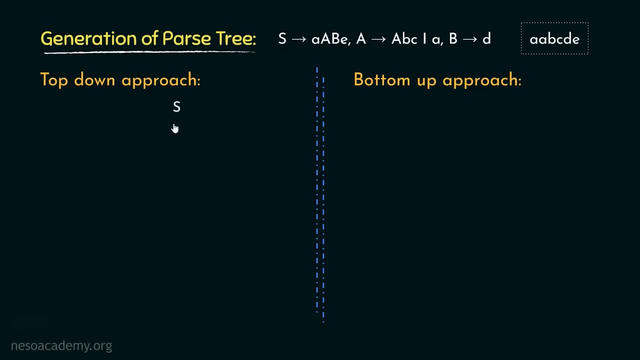 we are to generate the string a, a, b, c, d, e. Now, in case of the top-down approach, we will begin from the start symbol. So first we will take the start symbol. Now observe the production for S. S can be rewritten as small. a followed. 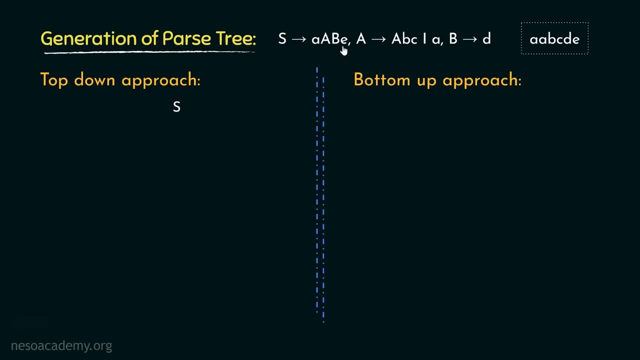 by capital A, capital B, followed by small e. So from S we will derive small a, capital A, capital B, small e. Now observe the string carefully. This particular string has a at the beginning and e in the end. Now, with this derivation we have covered the first. 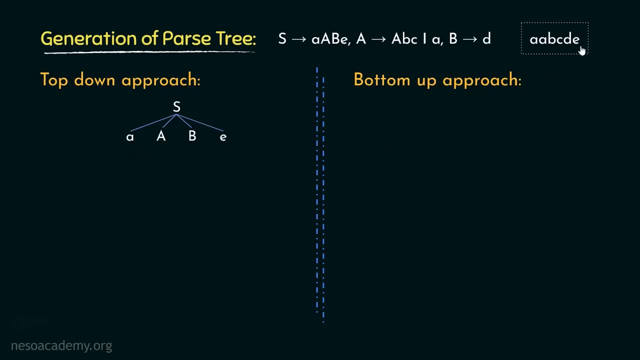 and the last e of this particular string. Now, coming back to our parse tree, we have got two more non-terminals, capital A and capital B. Let's observe the productions for them. A can be rewritten as capital A, followed by small b, small c or A can be rewritten as small a. Now coming to 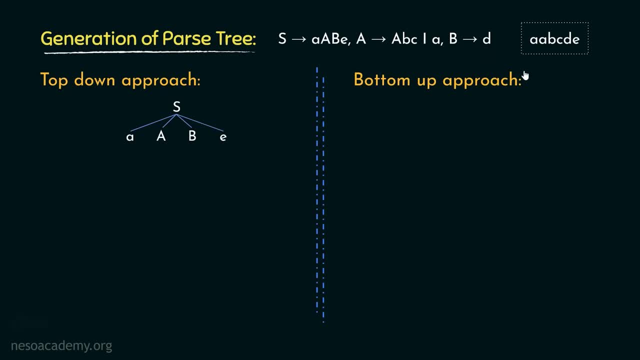 B. B can be rewritten as small d. Now observe the string a little bit more carefully. Apart from A and E at the beginning and at the end, we also have BC in the middle right. So if from this particular A, using the production rule, A can be written as ABC, we derive capital A, followed by 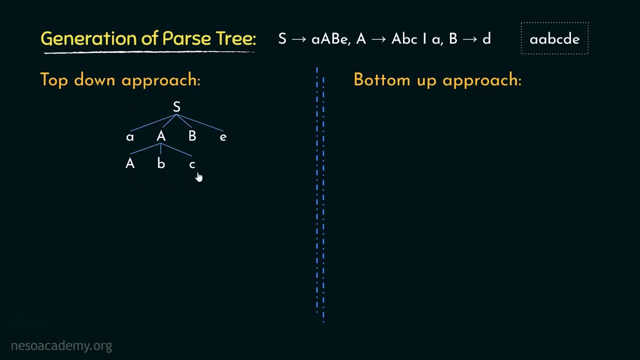 small b, small c. Now observe the derivation. Apart from A and E, we have now also covered the terminals BC in the middle of the string. Now let's come back to our parse tree. Observe from this: A selecting the production rule. A can be rewritten as A if we derive A With this derivation. 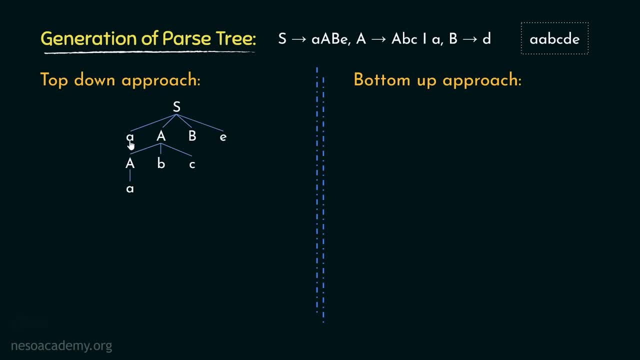 we have covered AA at the beginning. Observe A, then this A. Now, in this entire parse tree, we have got only one non-terminal, that is B, and B can be rewritten as d, So let's derive that from this B. that is terminal d. Now observe the yield AABCDE, which is exactly the same as B. Now let's. 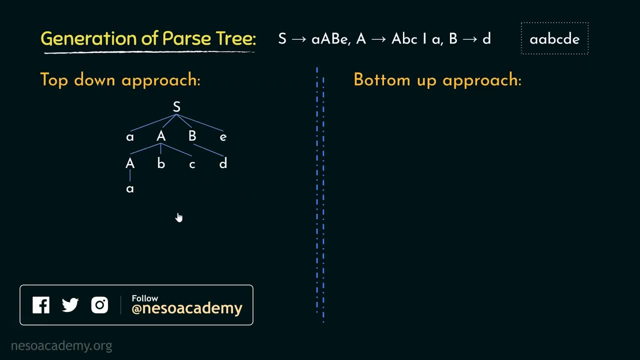 see how this string can be derived. So we will start off with A, followed by capital A, capital B, small e. Now, from this sentential form, we are going to select this A for expansion. Observe the parse tree. This A was expanded using the production rule: capital A, followed by small b. 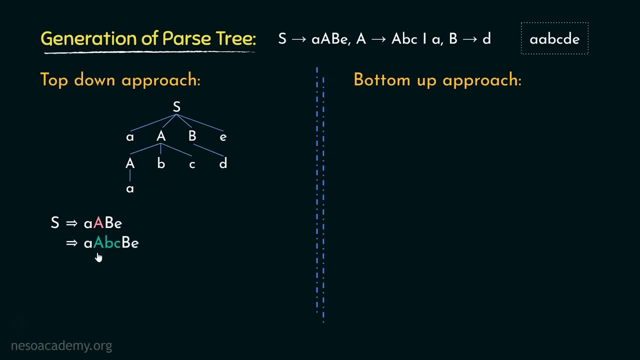 small c. So let's do that in here. Basically we use the production rule A, followed by capital B, small c. Now, coming back to our parse tree, observe Once this one is derived. after that we are going to expand this A, So we will select this A for expansion And from this A using the 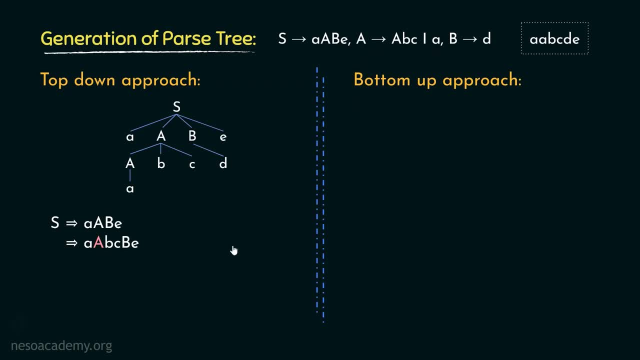 production. rule A can be rewritten as small a. we are going to derive small a Now in this entire string. this is the only non-terminal And the rule for that is B can be rewritten as d, So we will select this B for expansion And from this one we will derive d. Now observe this. 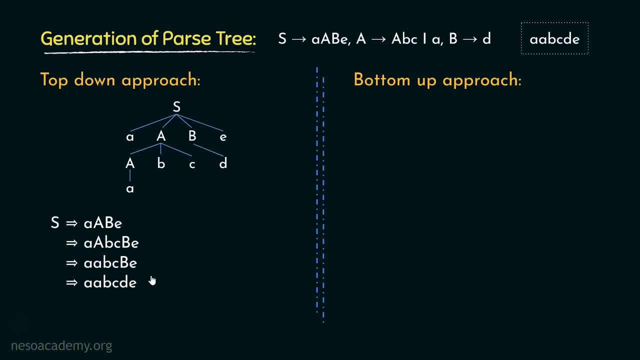 derivation carefully. At every point, we kept on expanding the leftmost non-terminal, didn't we? So this is leftmost derivation. So what I am trying to say is, in top-down approach, we use leftmost derivation. Now, during this derivation, the only decision we are going to make is 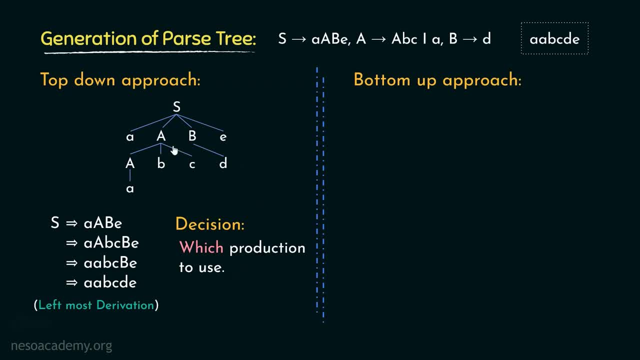 which production to use. Observe: From this A we could have derived A, But if we did so we couldn't derive Bc, And that is the reason we chose this production over this production. So basically, in top-down approach, 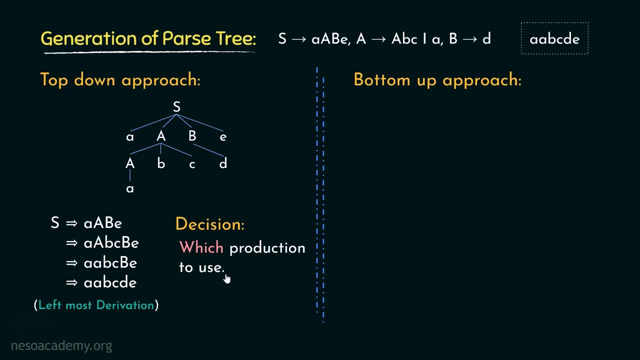 we are to decide which production to use at which step. So this is all about the top-down approach, which is followed by the top-down parsers. Let's now observe the bottom-up approach. As the name suggests, we will start off with the string itself Now, if you observe the production, 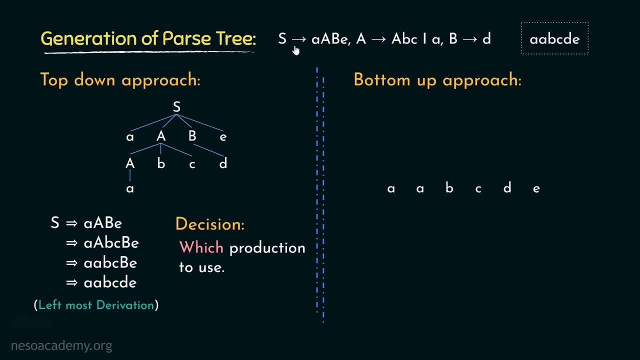 rules. we generally say the left-hand side can be rewritten as the right-hand side right, But alternatively we can also say the right-hand side can be reduced to the left-hand side, That is, this particular terminal D can be reduced to this particular non-terminal B. Using this logic, 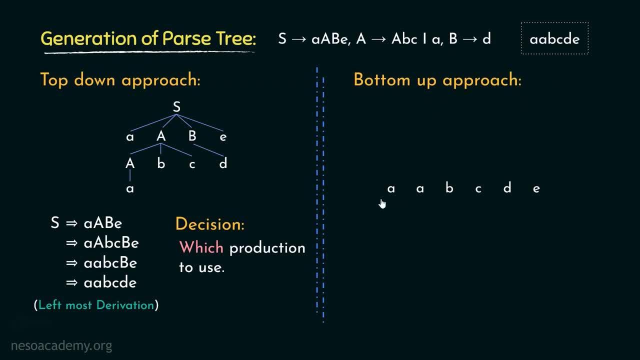 the bottom-up approach works. We will start off with the string itself And, using the production rules, we will keep on reducing the string until we get back to the start symbol. Let me show you how we do this Now in this particular string. 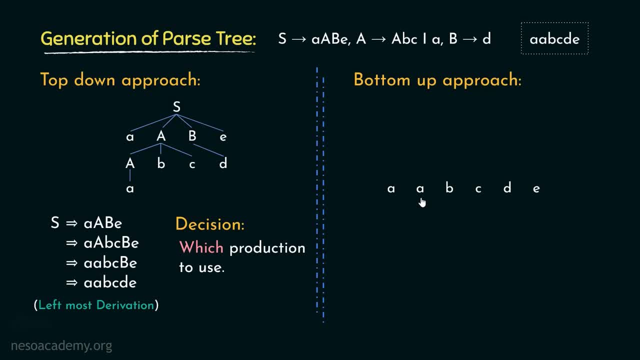 observe this: A. This A can be reduced back to capital A Using the production rule. A can be rewritten as small a, Or in other words, small a can be reduced to capital A. Now, after this is reduced to A, if we include A, B, C, these three can also be reduced to A, because capital A followed by B C can. 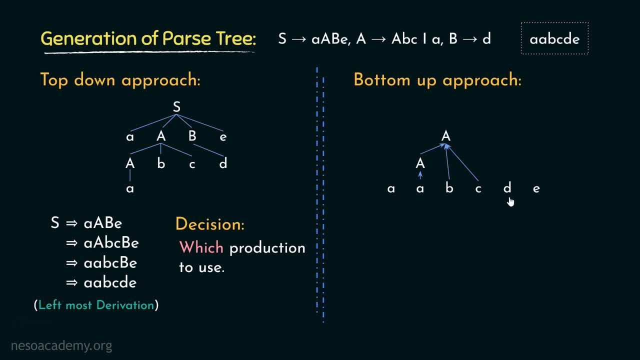 be reduced to capital A. Now observe, we have got this D, haven't we? Now? from the production rule, B can be rewritten as D, Or in other words, the terminal D can be reduced back to the non-terminal B. So let's reduce D back to B. Now observe, we have got A, followed by capital A, capital B. 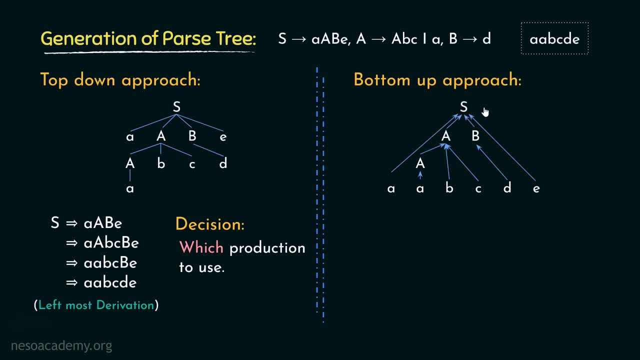 small e. Now all of these together can be reduced back to the start symbol S. Due to the production rule, S can be rewritten as small a, followed by capital A, capital B, small e, Or in other words the left-hand side of this production, can be reduced back to the start symbol S. 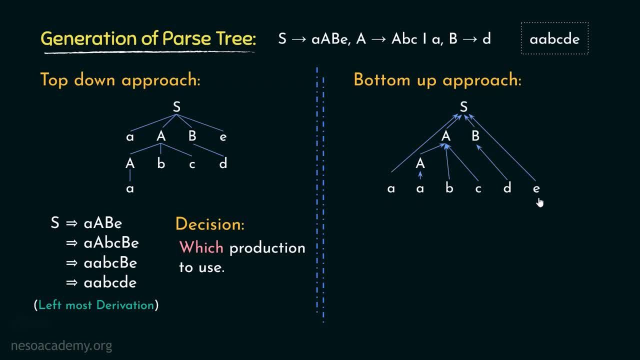 So, in bottom-up approach, starting from the string, we keep on reducing until we reach the start symbol, And this is how the parse tree is generated in B. Now let me illustrate this derivation in a linear manner, Starting with the start symbol S. 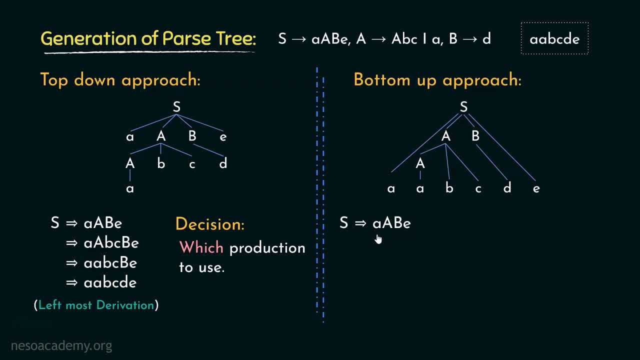 we are going to derive this sentential form: small a, capital A, capital B, small e. Now, this time we are going to select this B for expansion using the production rule. B can be rewritten as D, And from this B we are going to derive D. Observe: 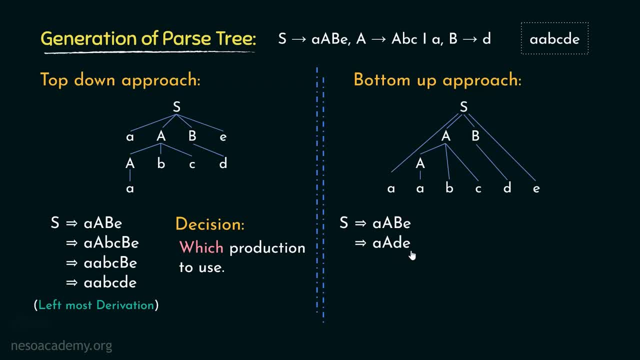 now, this is the only non-terminal in this entire sentential form, So we will select this non-terminal for expansion, And this time we are going to make use of the rule. A can be rewritten as capital A, followed by small b, small c. So from this A 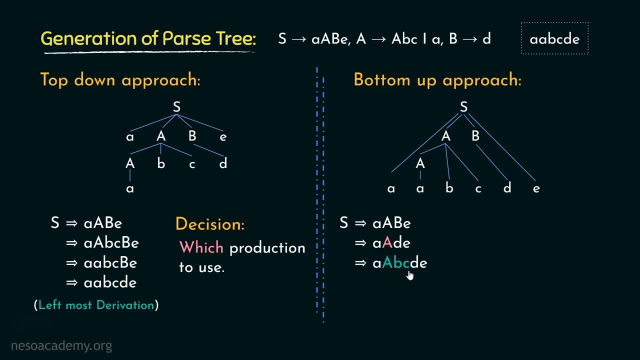 we are going to derive capital A, followed by small b, small c. Now observe: in this particular sentential form, this is the only non-terminal, So we will select that for expansion. Now, from this A we are deriving small a using the production rule. A can be rewritten as small a. 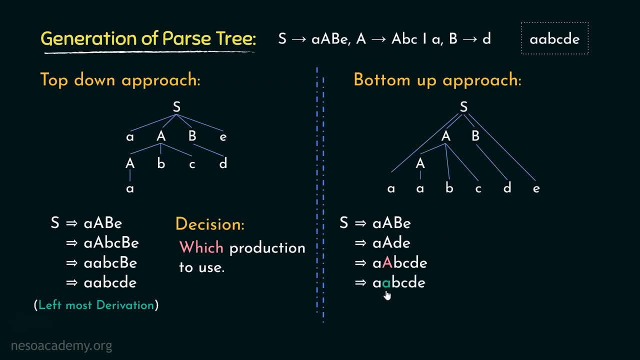 So from this A we are going to derive A. only Now, observe the derivation bit carefully. Starting from the first sentential form, at every point we kept on expanding the rightmost non-terminal, Isn't it? Therefore, this derivation is nothing but rightmost derivation. However. 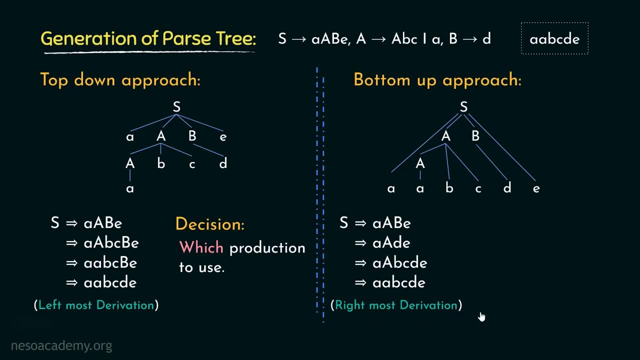 this is not exactly rightmost derivation, Now why so? Observe the bottom-up approach carefully. We didn't derive the string from the start symbol. Rather, starting from the string, we reduce the entire thing back to the start symbol. Therefore, it is rightmost derivation, but in reverse. So bottom-up approach. 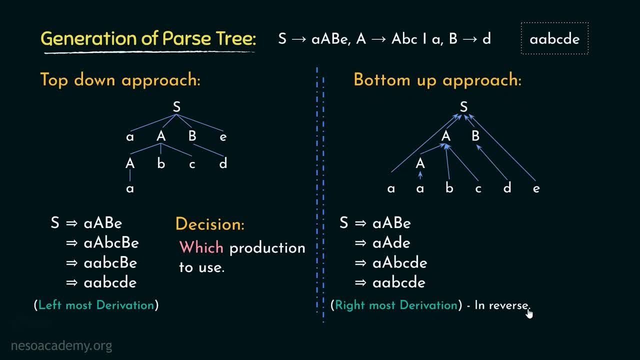 uses rightmost derivation in reverse And during the generation of this parse tree in bottom-up approach. the decision we are going to make is when to reduce. So this is all about the bottom-up approach, which is used by all the bottom-up parsers. So basically, the generation of parse. 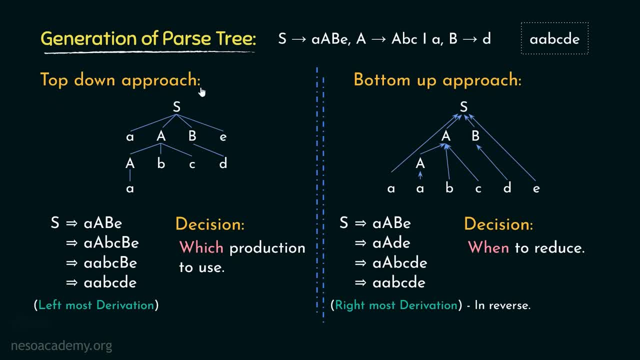 tree can be done in two ways. One is top-down approach, which is followed by the top-down parsers, And the another one is bottom-up approach, which is followed by the bottom-up parsers. Let's now observe the classification of parsers. So parsers can be broadly 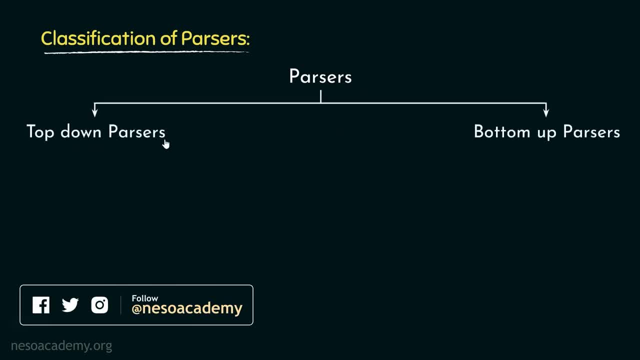 classified into two different categories: The top-down parsers, which use the top-down approach, and the bottom-up parsers, which use the bottom-up approach. Now coming to top-down parsers, these can be broadly classified into two more categories, That is, top-down parsers with backtracking and top-down parsers without backtracking. 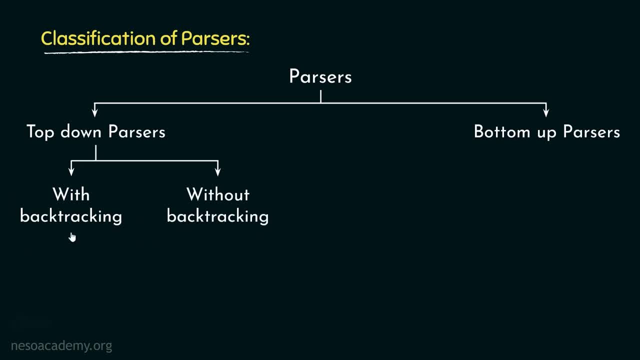 Now the top-down parsers which allow backtracking can be categorized into brute forcing algorithms And this particular top-down parser uses the method of backtracking which we observed in the session: Non-determinism in CSGs Coming to the top-down parsers without backtracking. 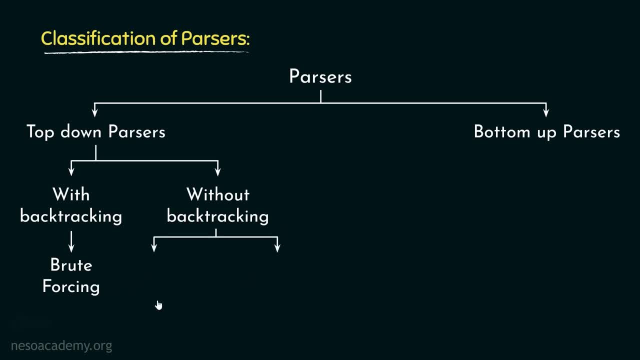 This can also be further classified into two different categories. One is the recursive descent parsers And the next one is the predictive parsers. Now, some examples of predictive parser are LL1, LLK. Now coming to the bottom-up parsers, these are also known as the shift reduce parsers. 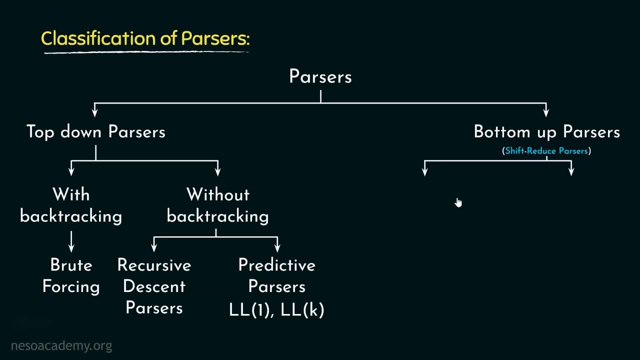 Now these parsers can also be classified into two different categories, into two different categories. one is the operator precedence parsers and the other one is the LR parsers. now coming to LR parsers, these can be classified into four different categories: LR 0, SLR 1, LLR 1 and CLR 1. now we will learn. 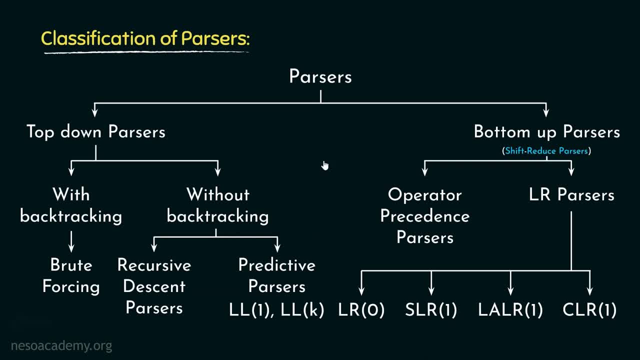 about the different parsers in different sessions. in this chapter we are going to focus on the top-down parsers, specifically the top-down parsers, without backtracking, and in the next chapter we will learn about all the bottom-up parsers. however, I would like to provide some insights about the